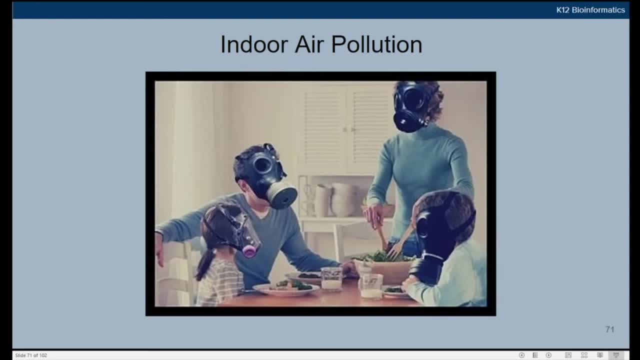 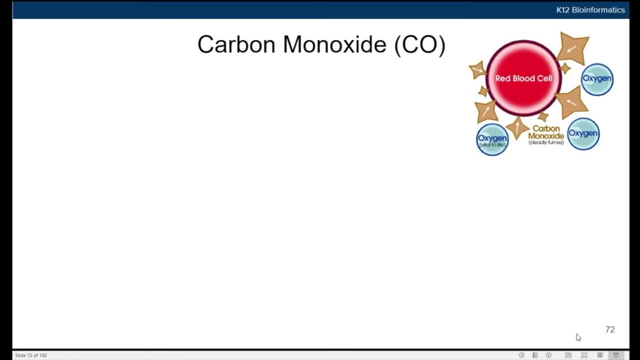 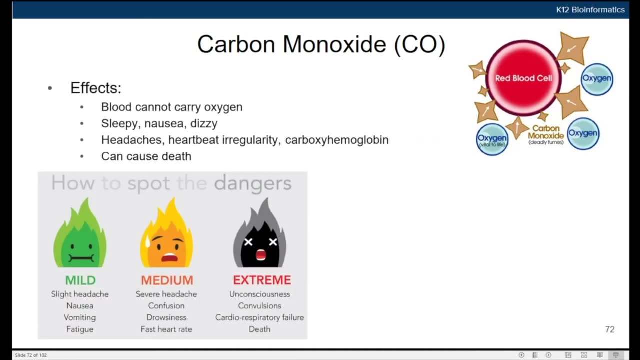 Our fifth subunit on the exposome focuses on indoor air pollution. We discussed carbon monoxide in the last unit, but it's worth a closer look, considering how dangerous it is. as an indoor air pollutant, Carbon monoxide binds to red blood cells, preventing oxygen from binding. This means 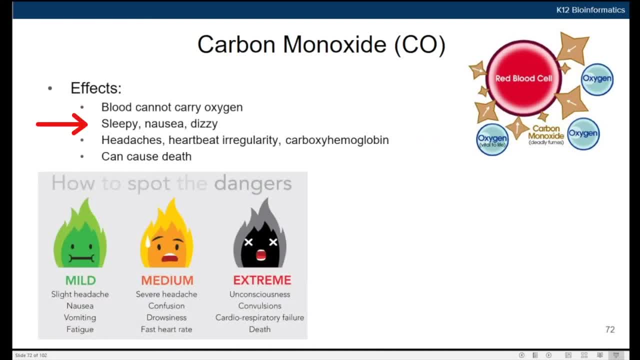 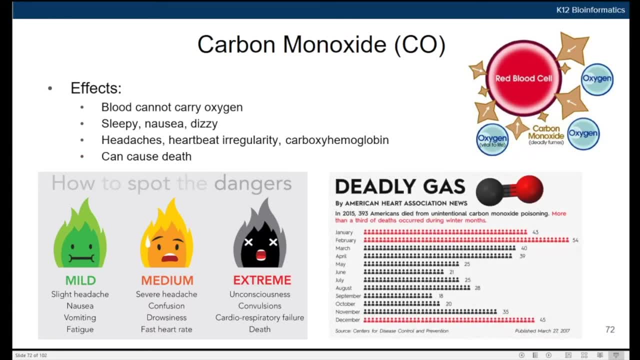 that the blood can't carry oxygen, which leads to sleepiness, nausea, dizziness, headaches, heartbeat irregularity and carboxyhemoglobin, which can lead to death. Deaths attributed to carbon monoxide poisoning tend to increase during the winter months, presumably due to increased 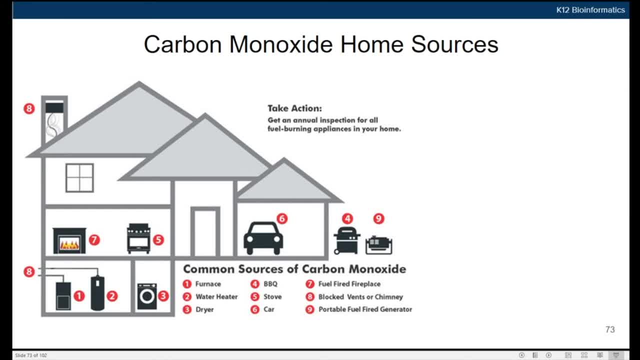 combustion, heating and homes. This figure illustrates potential sources of carbon monoxide in the home. Given that it can't be seen, smelled or heard, it's important to install carbon monoxide detectors so it can be stopped. And, of course, it's important for people to be aware of the signs. 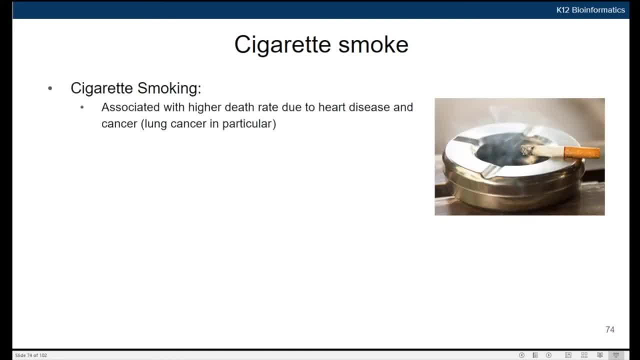 of carbon monoxide poisoning. As previously mentioned, cigarette smoking is associated with higher death rates due to heart disease and cancer. It's considered to be the deadliest indoor air pollution in the world. It's also considered to be the deadliest indoor air pollutant. Cigarette smoke contains formaldehyde and carbon monoxide, in addition to particulates. 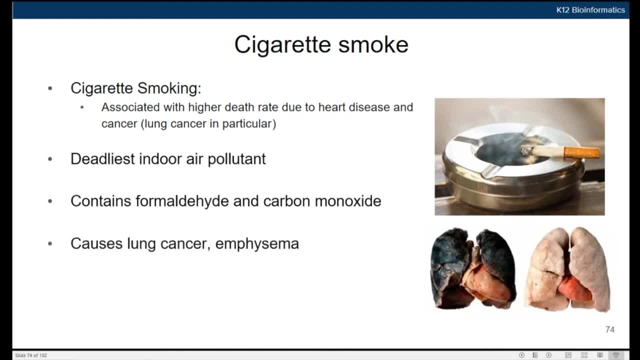 and other chemicals. It's been established to cause lung cancer and emphysema, and secondhand smoke may be even worse due to the particulates that come from the burning tip rather than smoking through the filter. Of note. it's not just cigarette smoke that can be harmful to human. 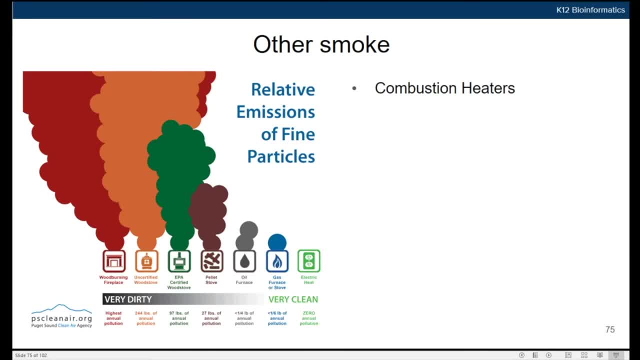 health. Home combustion heaters can release varying amounts of fine particulates into the air. This figure illustrates relative emissions of fine particles by different combustion heaters, from a wood-burning fireplace all the way to electric heaters, which are the cleanest with respect to indoor air pollution. You may not think of it. 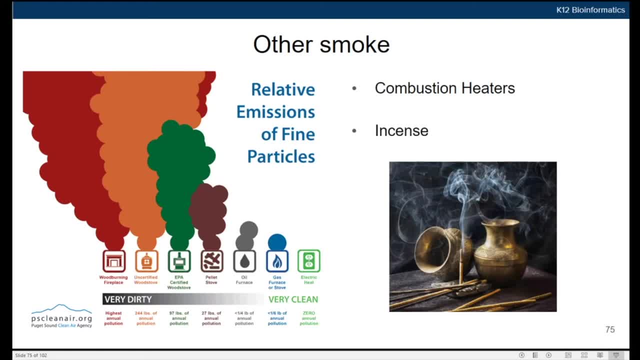 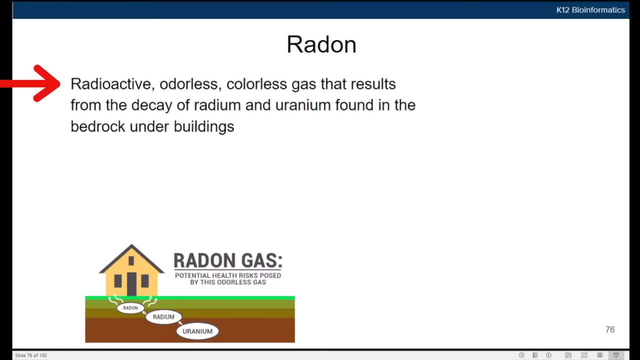 but even incense can be a harmful indoor air pollutant, given its release of fine particulate matter. Another well-known source of indoor air pollution is radon. Radon is a radioactive, odorless, colorless gas that results from the decay of radium and uranium found in the bedrock. 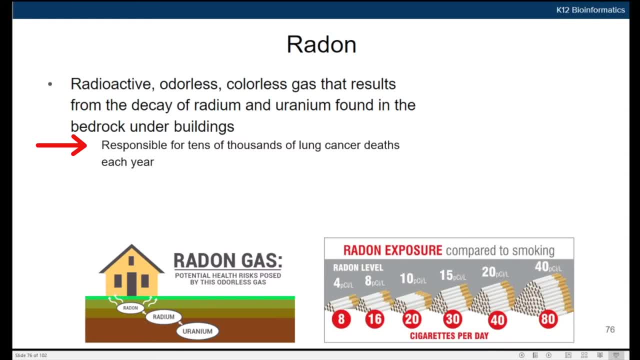 under buildings. Radon is responsible for tens of thousands of light years of air pollution. In this illustration, we can see how radon exposure can be compared to cigarette smoking in terms of its potential for negative health consequences. Radon exposure can be prevented by. 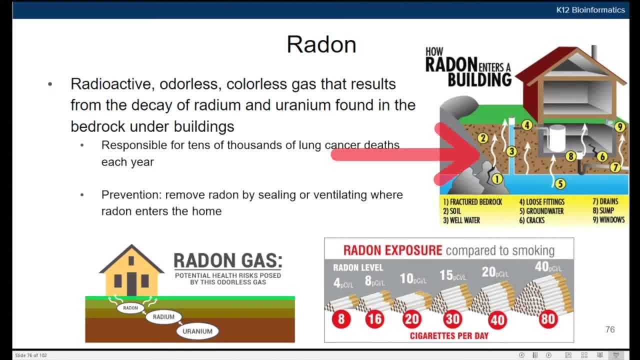 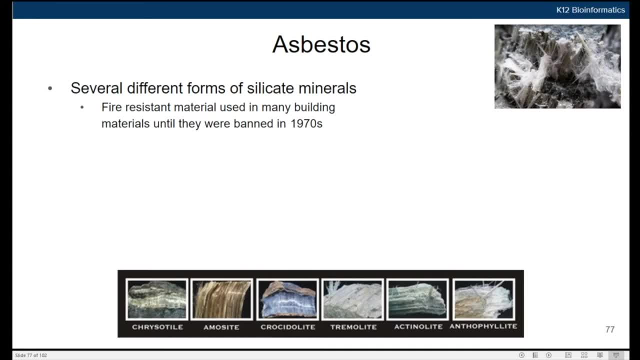 sealing off or ventilating spaces in the home where radon may enter, such as the basement Mentioned earlier. asbestos is another dangerous indoor air pollutant as a particulate. Asbestos is a set of different forms of silicate materials Due to their fire-resistant properties. 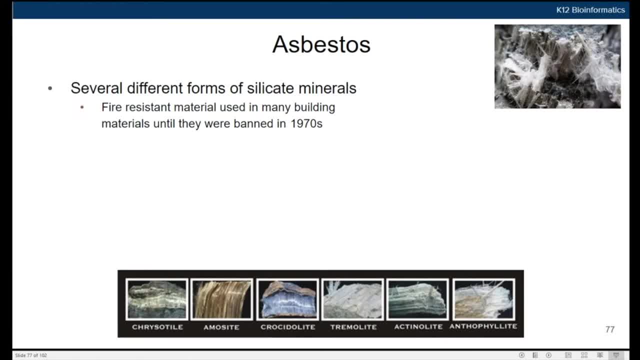 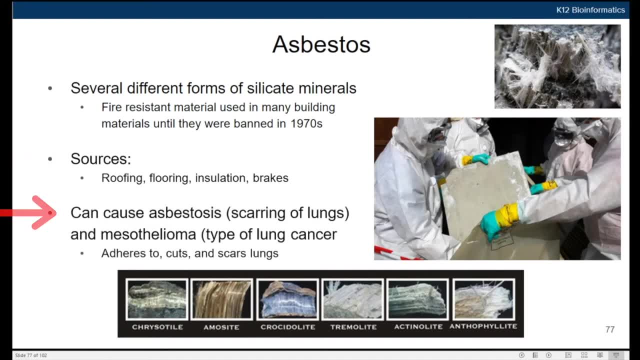 they were used in many building materials until they were banned in the 1970s. Asbestos can be found in the roofing, flooring, insulation or breaks of older buildings and vehicles. The inhalation of asbestos can cause asbestosis or the scarring of the lungs. 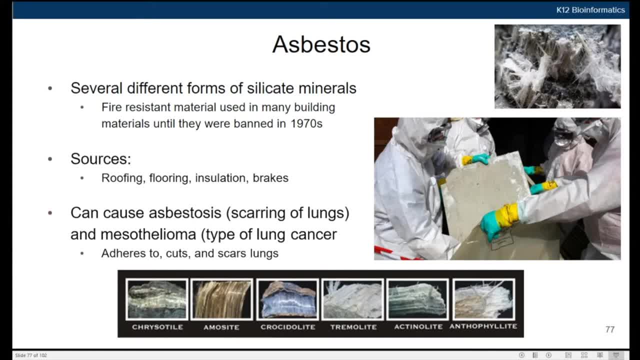 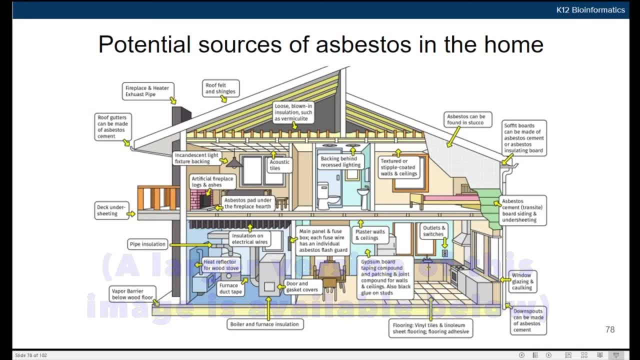 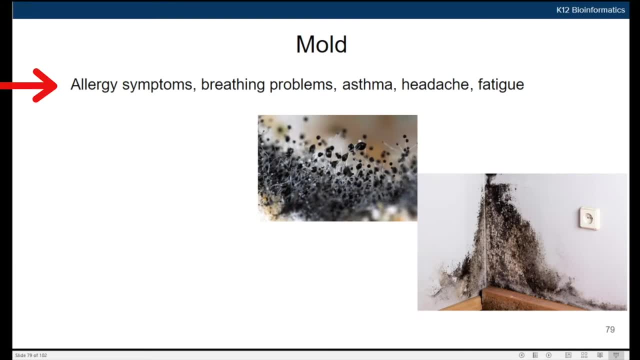 as well as mesothelioma, a type of lung cancer. This figure illustrates potential sources of asbestos in homes built in or renovated prior to 1989.. One biological indoor particulate pollutant asbestos is mold, which can lead to allergy symptoms, breathing problems. 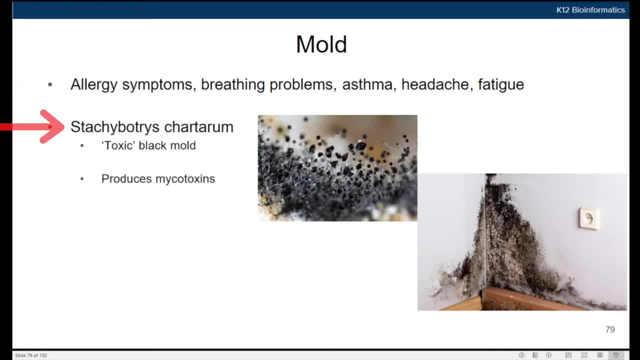 asthma, headache and fatigue. A particular variety of mold, known as black mold, produces mycotoxins. Black mold has a notorious reputation that has been exaggerated to some extent by the media. However, exposure to black mold can still bring about serious symptoms. 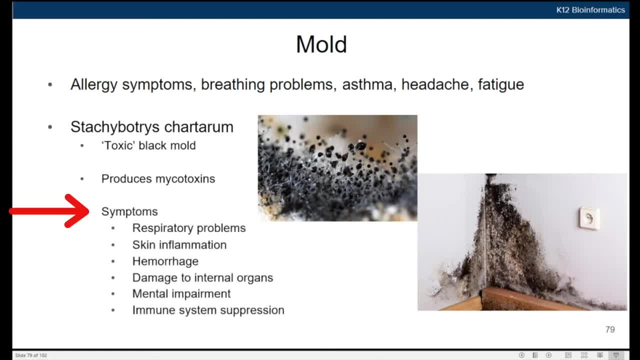 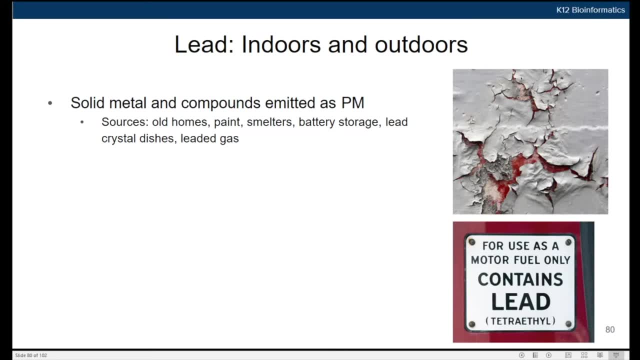 including respiratory problems, skin inflammation, hemorrhage, damage to internal organs, mental impairment and immune system suppression. Lead is one of the criteria pollutants measured by the EPA monitoring stations and is a serious concern both as an outdoors and indoors air pollutant. Lead presents an air pollution risk as particulate matter. 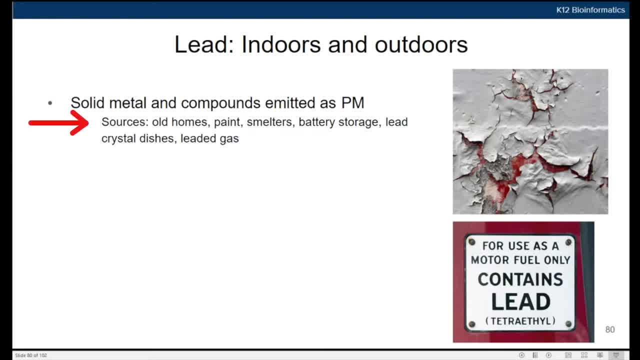 with sources including old homes, paint smelters, battery storage, lead crystal dishes and leaded gas. An estimated 2 million tons of lead enter the atmosphere every year. The health impacts of lead include an accumulation in tissues which affects the kidneys, liver and nervous system. 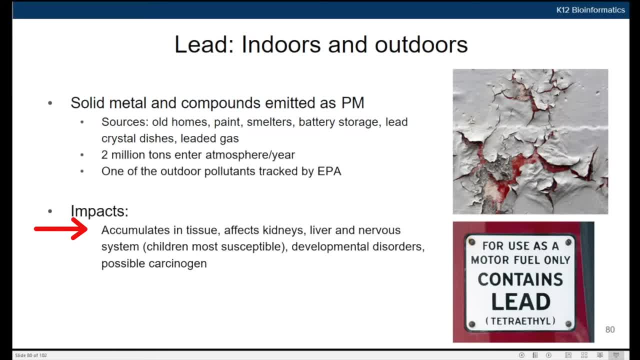 with children being exposed to lead every year. Lead can also be used to treat diseases and is a potential carcinogen. Lead is also known to cause behavioral and learning problems, slow growth, hearing problems and headaches. Another air pollutant that is of great concern, both outdoors and indoors are volatile organic. 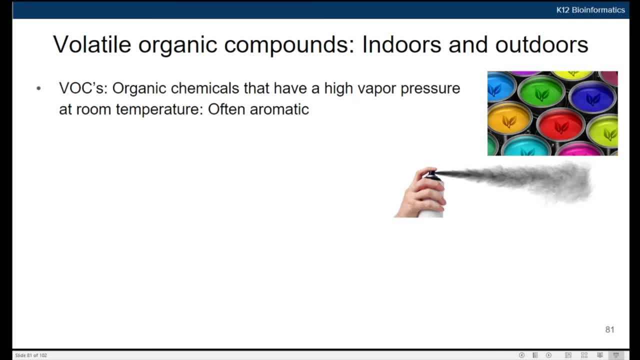 compounds or VOCs. You might recall earlier we mentioned that VOCs are a chemical precursor to bad ozone. VOCs are organic chemicals that have a high vapor pressure at room temperature and often, but not all, are harmful to the environment. They can be harmful to the environment and can cause 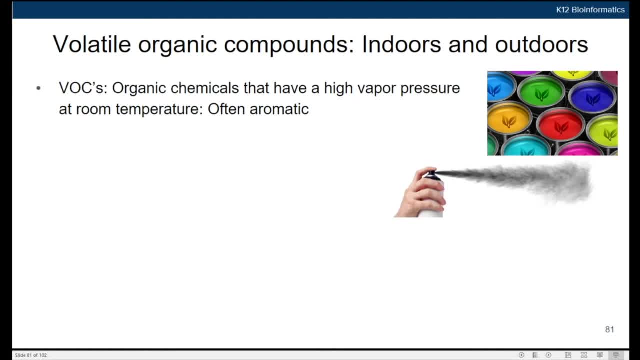 damage to the environment. VOCs can be categorized as either methane or non-methane VOCs. Methane is an extremely efficient greenhouse gas which contributes to climate change. Some examples of aromatic non-methane VOCs include benzene, toluene and xylene. It's typical to expect 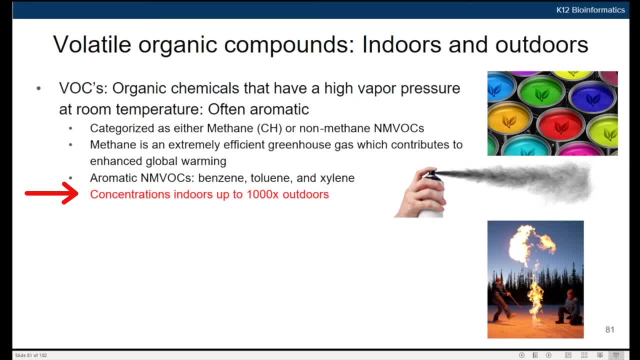 VOC concentrations indoors up to a thousand times higher than those observed outside. VOCs can be released by building materials, indoor furnishings, glues, adhesives, printers and copiers, mothballs, insecticides and dry cleaned clothes. Towards health, VOCs can irritate eyes and the respiratory system. they can be carcinogenic. 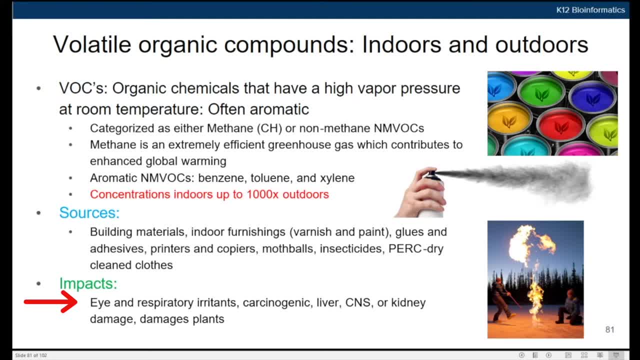 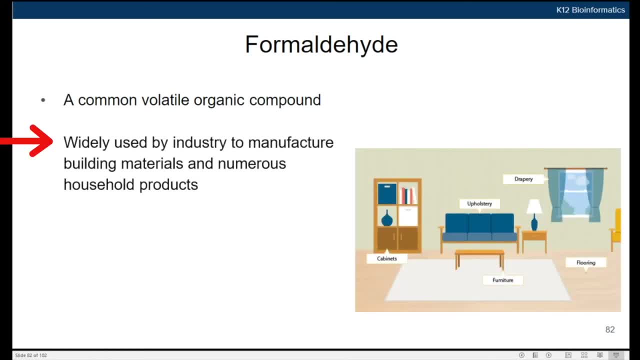 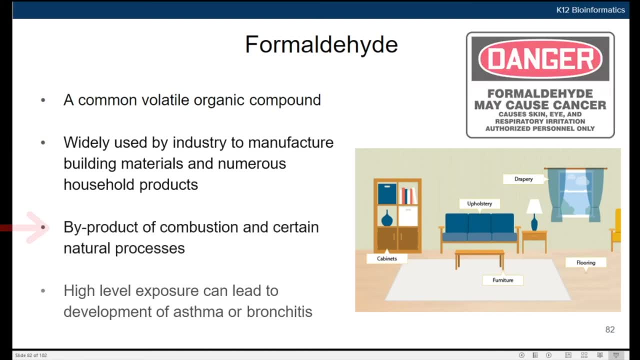 and can cause liver, central nervous system or kidney damage, as well as damaged plants. One particular VOC worthy of additional focus is formaldehyde. Formaldehyde is used widely in industry to manufacture building materials and numerous household products. It is a byproduct of combustion and certain natural processes. High level exposure can lead to the development of. 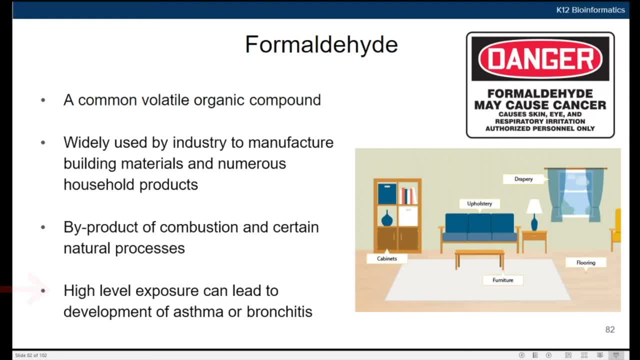 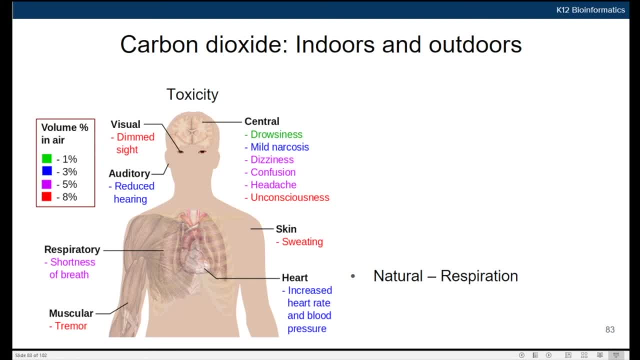 asthma and bronchitis, as well as being a potential carcinogen. We'll look at carbon dioxide. Even the product of our own respiration can be thought of as an air pollutant, since high levels can lead potentially to long-term health health. 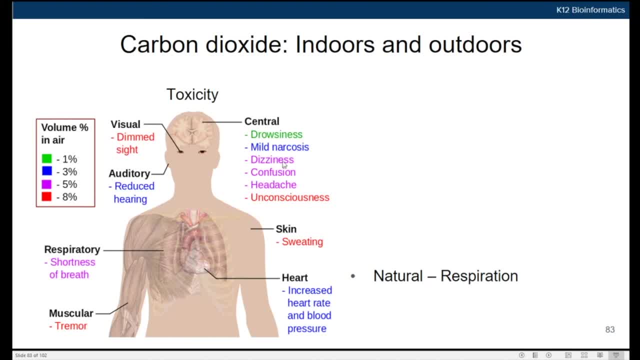 consequences. This figure lays out some of the symptoms of carbon dioxide levels in the air. At 1 percent, carbon dioxide leads to drowsiness. At 3 percent, carbon dioxide can lead to reduced hearing, mild narcosis and increased heart rate and blood pressure. 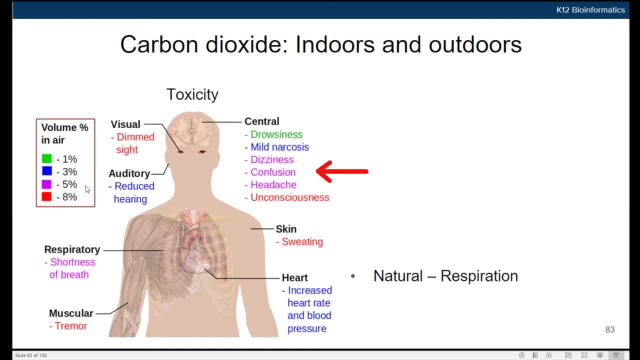 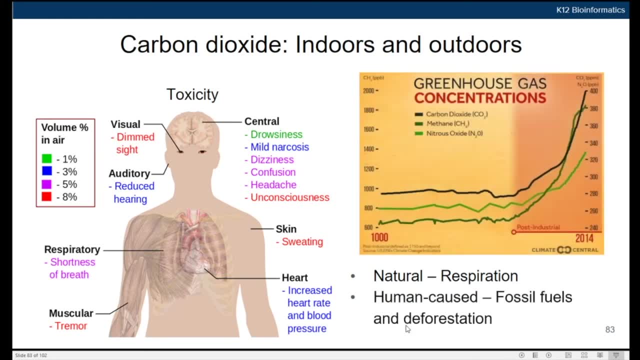 At 5 percent, shortness of breath, dizziness, confusion and headache are introduced, and at 8%, there can be tremors, dimmed sight, sweating and unconsciousness. Outdoor carbon dioxide levels can also increase by the burning of fossil fuels and deforestation. Carbon dioxide is, of course, one of the greenhouse. 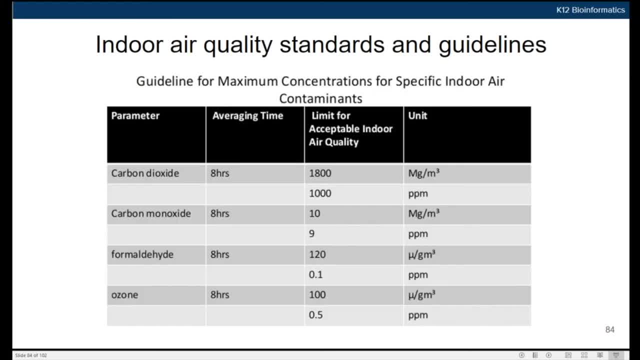 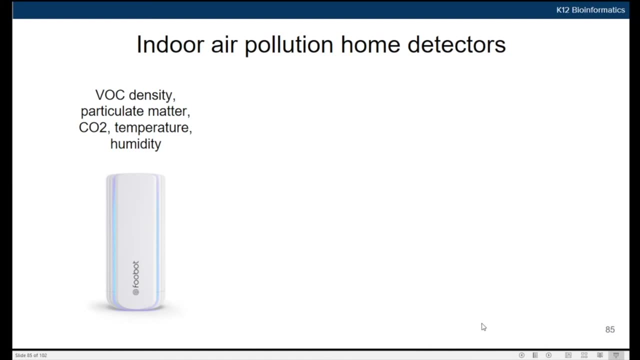 gases that has been associated with climate change. Standards for the maximum concentration of specific indoor air contaminants have also been proposed, but obviously less is always better for any of these. There are, of course, detectors to warn of risky levels of specific indoor air pollutants, the most common of which is the smoke and carbon monoxide detectors. Radon detectors are 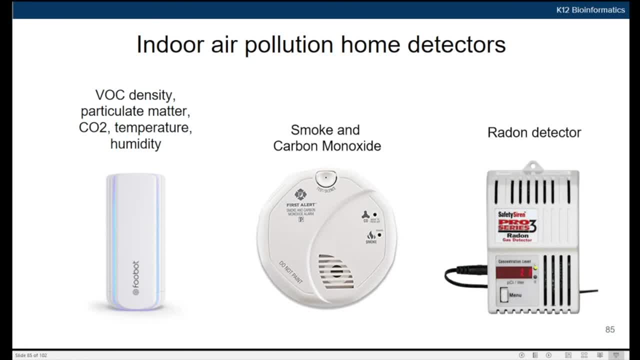 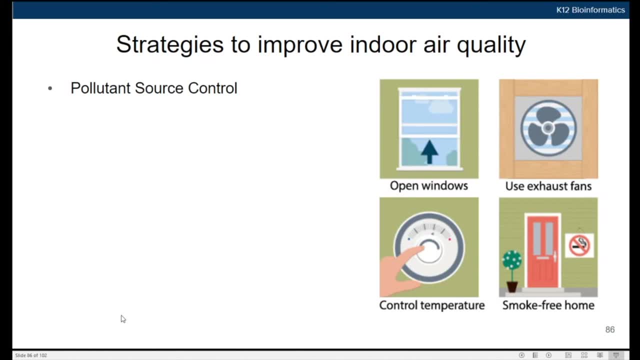 also common in some parts of the country. However, it is still uncommon to monitor many other common sources of indoor air pollution. So what are some strategies to improve indoor air quality? For one, we can seek to control pollutant sources. An example of this might be banning smoking within